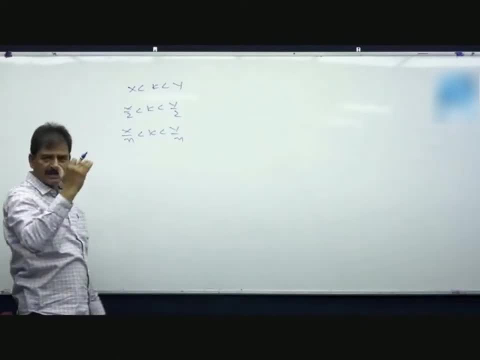 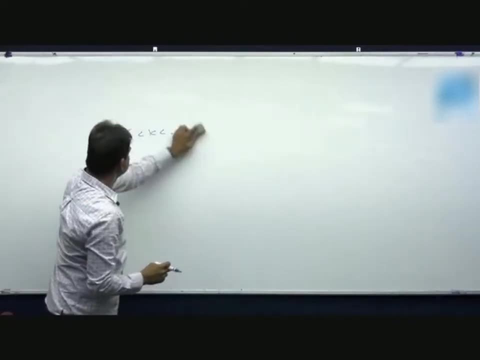 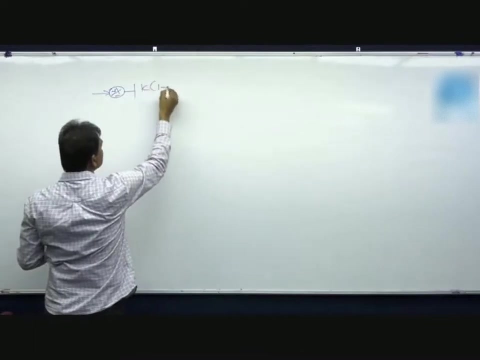 by n For every loop, the range of k reduces. For three loops it becomes x by 3 less than k less than y by 3.. For example, if you take example, a simple example, let us take up. For example, it is like this: k into 1 minus s by 1 plus s, If you find the range of k for 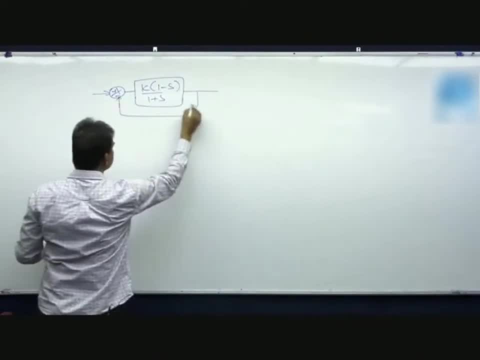 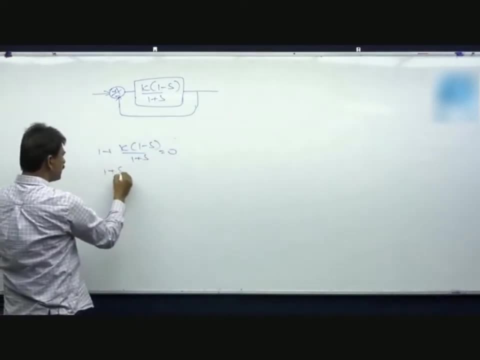 stability with this. with one loop, 1 plus k into 1 minus s. by 1 plus s, This is equal to 0.. 1 plus s plus k minus k s is equal to 0.. Here, 1 minus k into s 1. 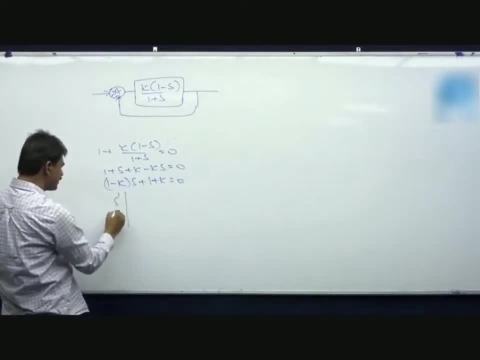 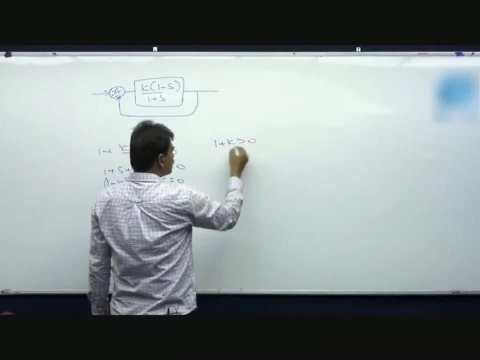 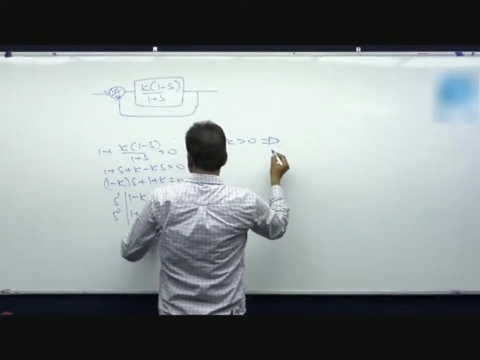 plus k 0.. Therefore, simple tabulation: s power 1, s power 0, 1 minus k, 1 plus k. both should be greater than 0, greater than 0.. This gives k. This is going to give 1 minus k, 1 plus. 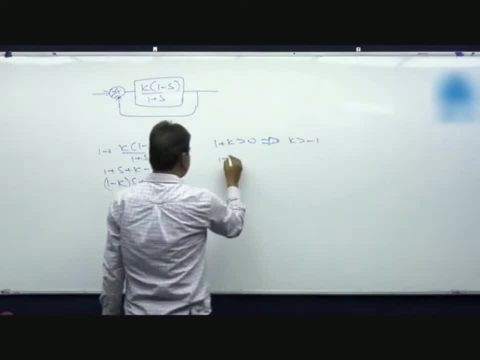 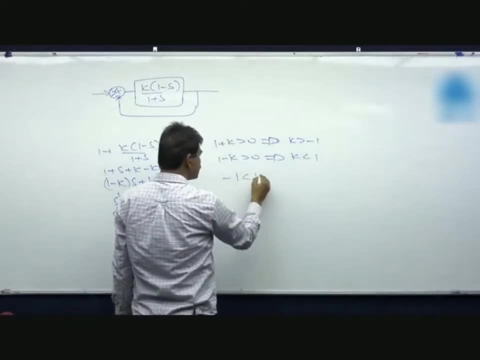 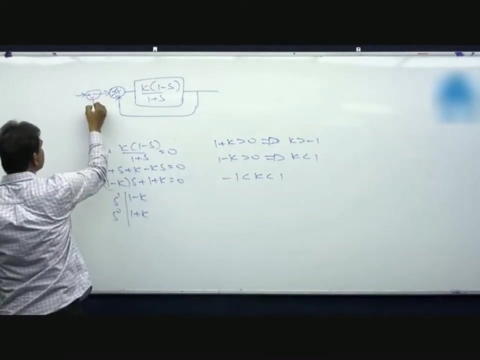 k k greater than minus 1.. 1 minus k greater than 0. This gives k less than 1.. Therefore, range of k is minus 1 to plus 1 with the inner loop If one more loop is connected like this and tested the stability. 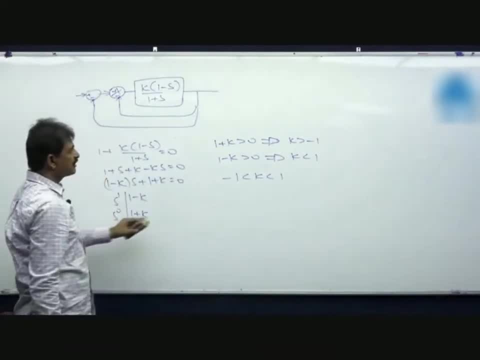 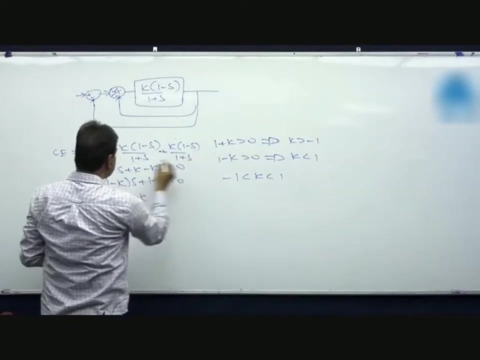 therefore now the range of k for stability becomes 1 by 2, less than k, less than 1 by 2.. Because here characteristic equation is 1 minus sum of the loop gains, There is one more loop, you will get it k into 1 minus s by 1 plus s. Therefore factor 2 comes here. 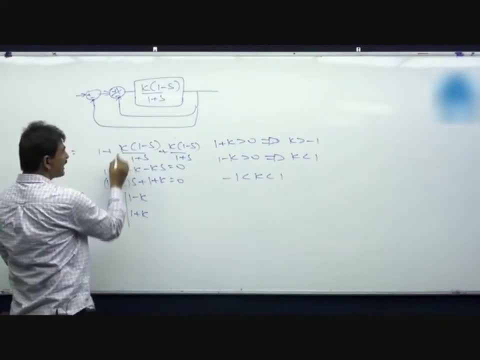 2 loops, 2 k factor. Therefore, everywhere k should be replaced by 2 k. Therefore 2 k comes here. You can verify here What is the characteristic equation now: 2 k into 1 minus s by 1 plus s. This is characteristic equation is 1 minus sum of the loop, gains plus sum. 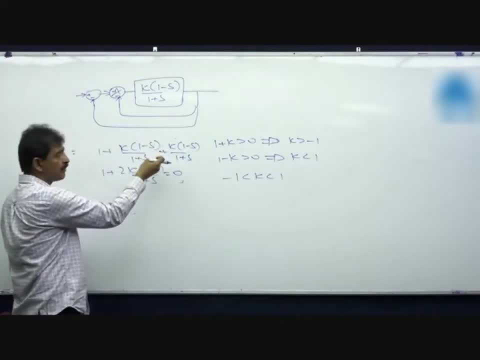 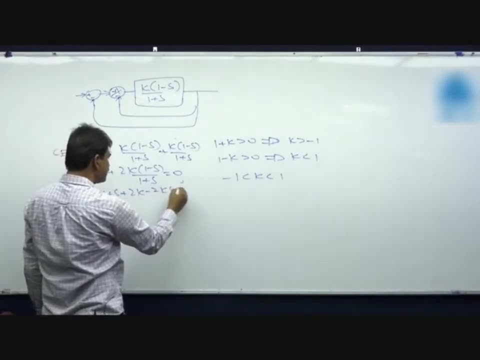 of the gain product of 2 non-touching loops. Mason's gain formula is denominator. Therefore, 1 plus s plus 2 k minus 2 k s is equal to 0.. Here you can see here, 1 minus 2 k into.